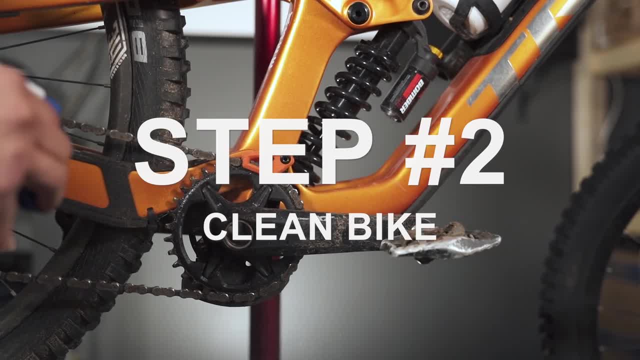 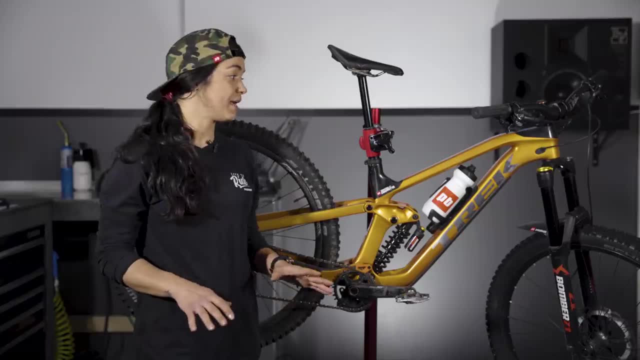 So black on black on black. Step two: start with a clean bike, because it's going to keep your workspace a lot tidier and you can really see what's going on with the bike under all the mud. I wash my bike, or at least rinse it down, after every ride in the winter. I. 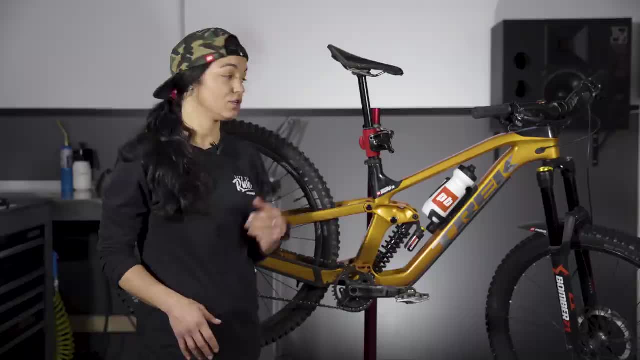 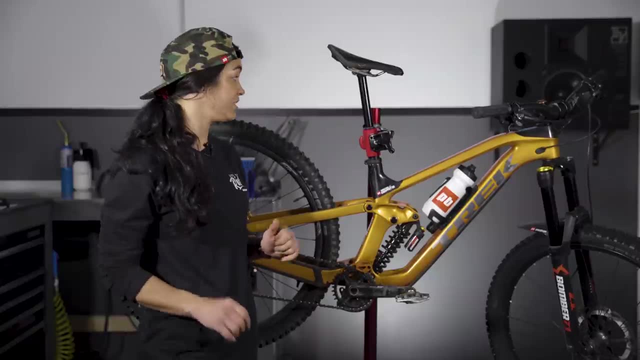 don't want the mud to get caked on there, stuck and frozen. So if you wash it when it's still a little bit moist, it's going to clean up really nicely, And if you're going to be using sand, you're going to want to be really careful about that. 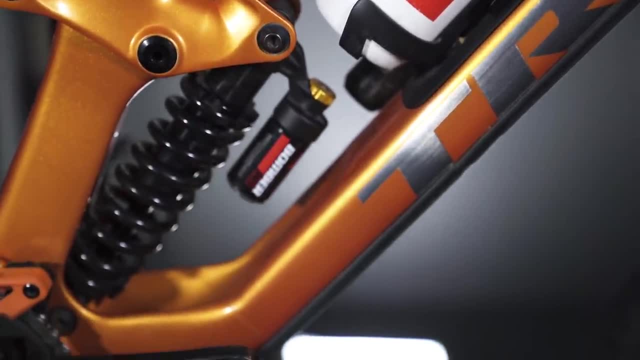 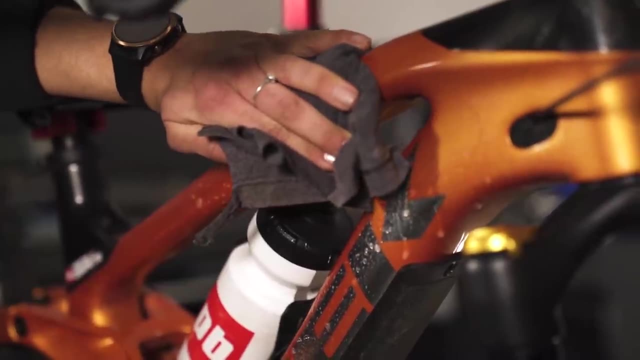 though. Be really cautious of all the seal locations and your bearings on the bike as well. You don't want to be pushing mud into those places, So a nice low setting on the hose will be really helpful there Once the bike's clean. I just like to give it a little. 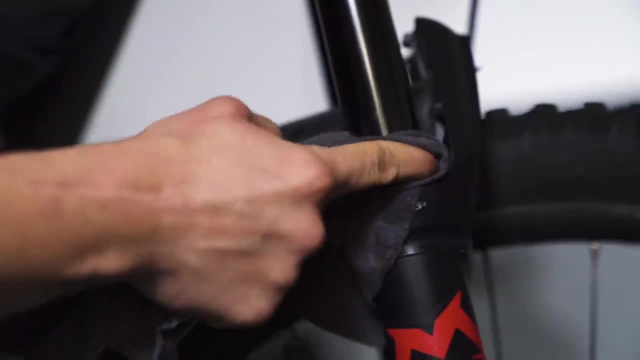 wipe down with a nice clean cloth, Get rid of all the mud that's still lingering around. And while you're there, it's a good idea to wipe the seals on your fork, as well as the seals on your dropper post, And if you have an air shock, do that as well. 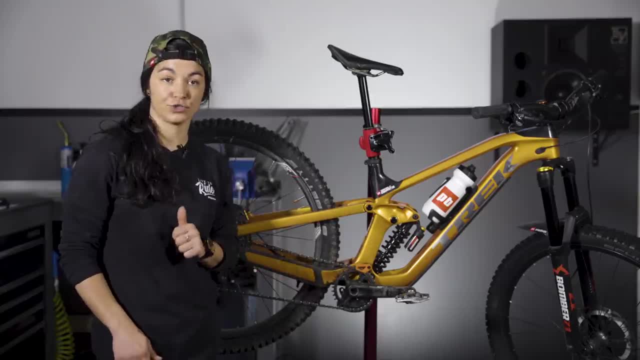 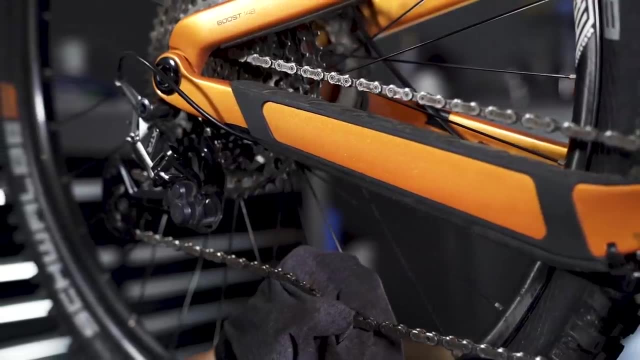 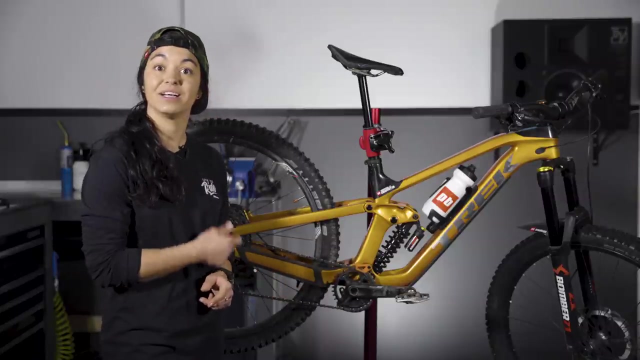 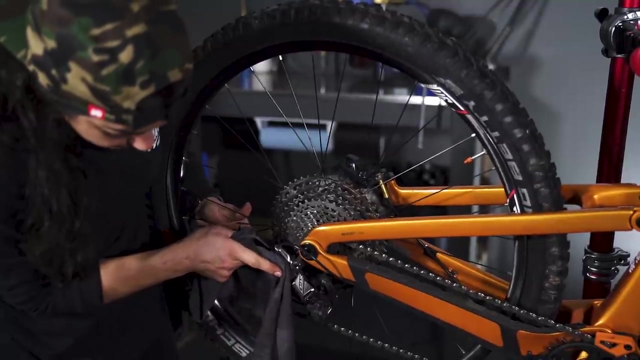 Before moving on to the rest of the bike, I like to first address the chain. Don't want to forget to lube the chain, to try to do it as soon as you've cleaned the bike, And now's a good time to get really up close and personal with your chain. You've always wanted to count how many chain links are in there, so count them up, Clean every single individual one, because the water and the grime that's stuck in between those little rollers, that's what's wearing the chain down very quickly and more prematurely than the rest of your drivetrain. 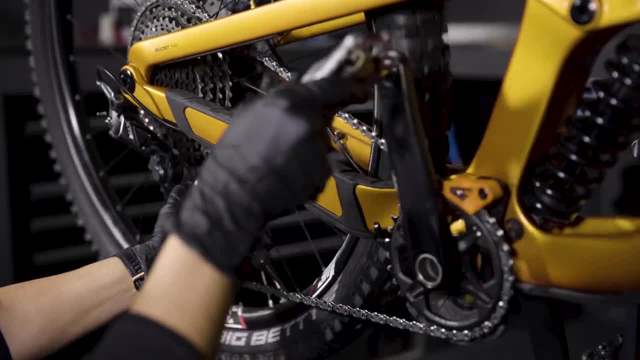 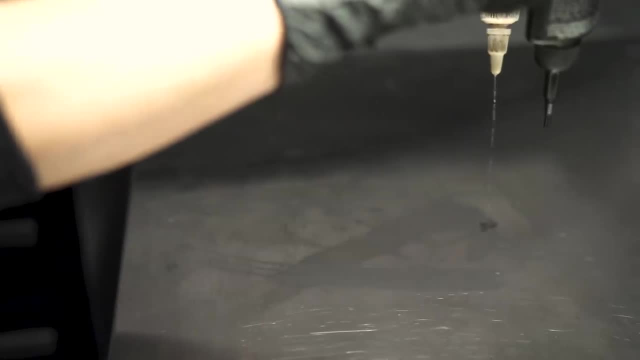 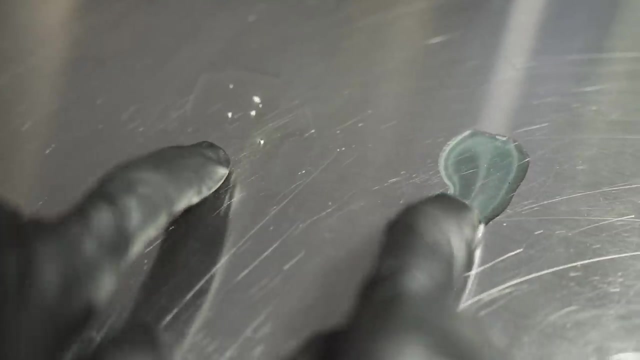 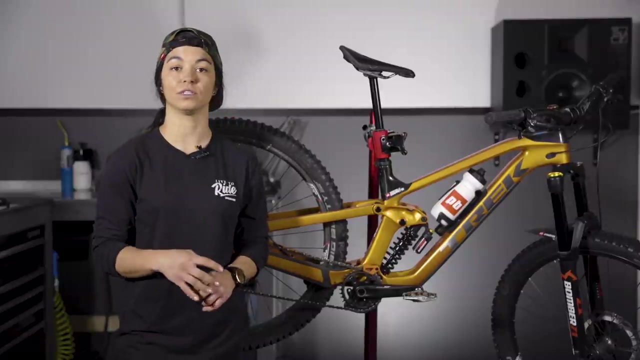 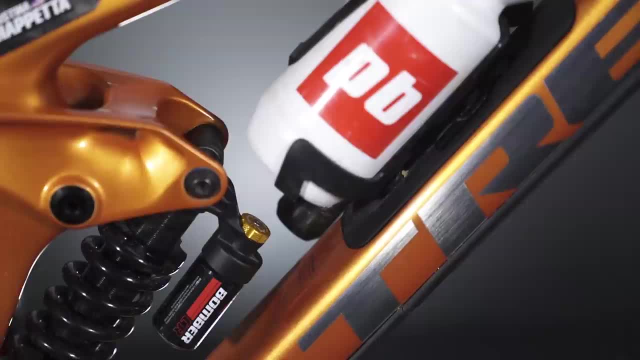 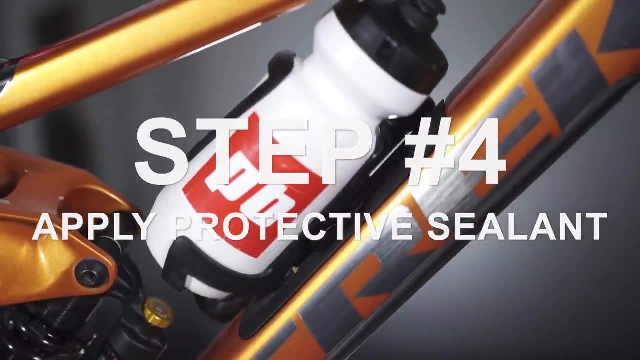 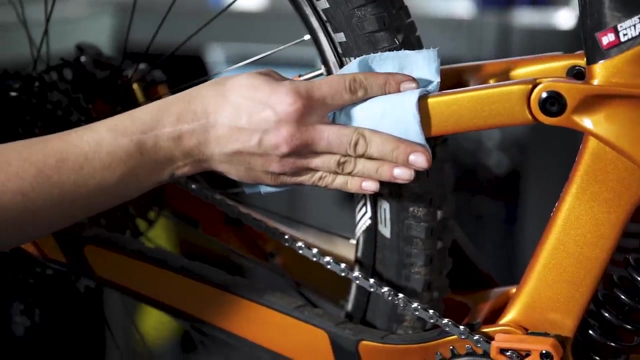 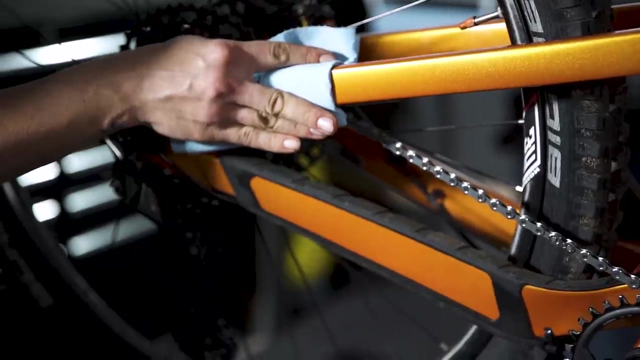 is just going to pick up grime and dirt and dust later on. Moving on, now that the bike looks nice and clean to the naked eye, here I like to use a little bit of protective sealant spray on the frame. That way, the next time you go out and ride, the mud and the water it's going to drip off a lot easier. But do be careful. You don't want to just go spray it free willy nilly all over the bike because guaranteed you're going to get it on the rotors and the brake pads and all the places you don't want the spray. So what I do instead is I apply it to a little bit of a clean rag and then just 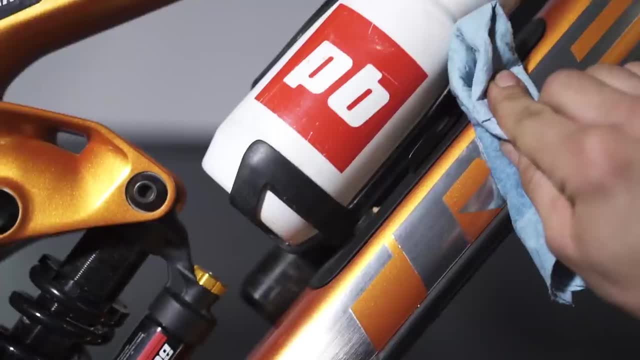 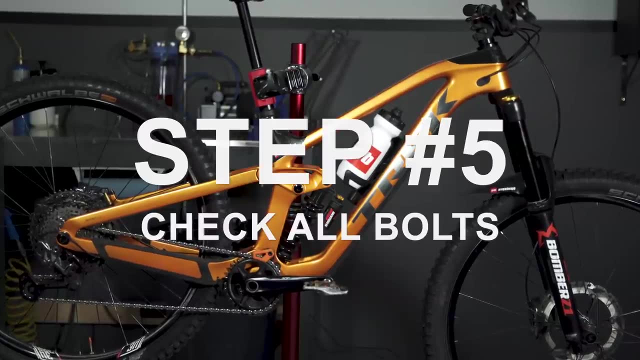 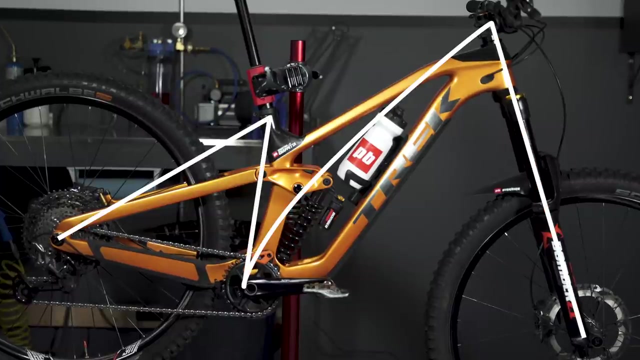 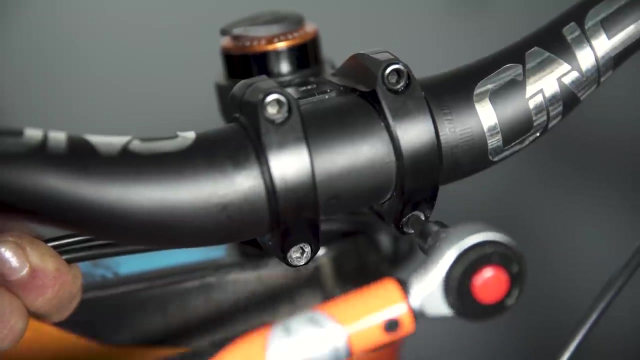 wipe it onto the bike, You pretty much get the same effect and it looks nice. We're finally ready to actually service the bike now. So what I do is a little helpful reminder for myself. to make sure I'm not missing any bolts is I do a little bit of an M pattern on the bike when I'm just going through checking the bolts? But do make sure to use a torque wrench, especially on the really fancy and delicate parts like carbon handlebars, frames, all those pieces that you don't want to over torque or else you're going to break something. 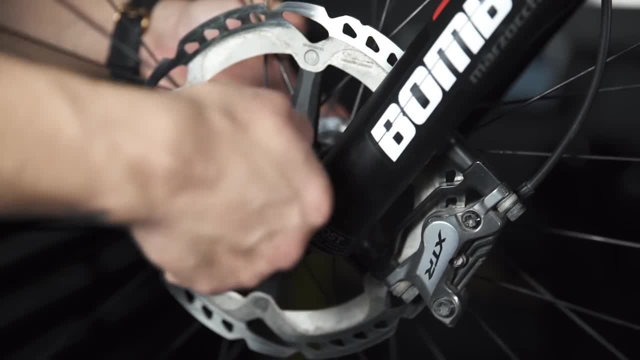 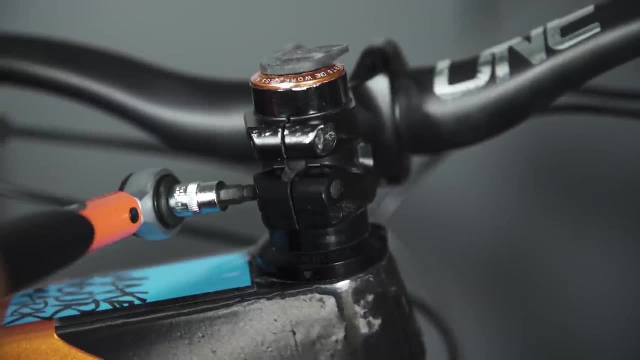 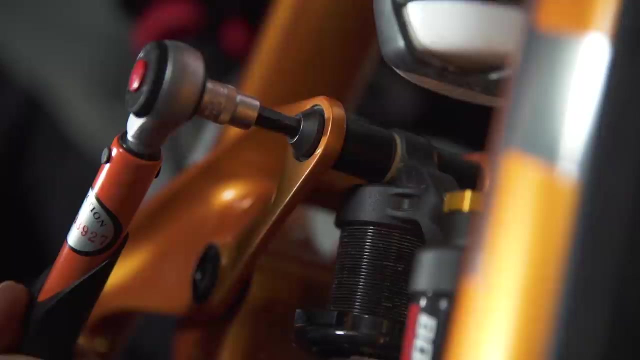 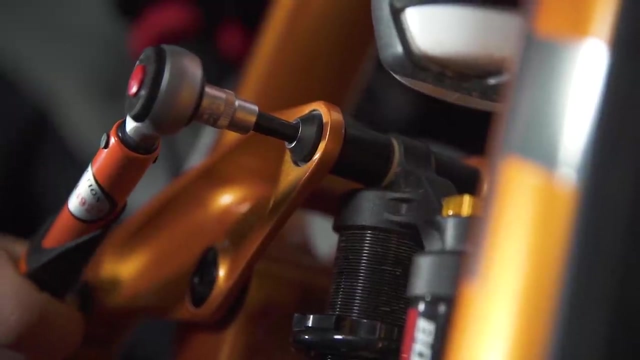 And those parts are quite expensive. Starting at the front, we're going to do the axles, the brake adapter, Moving up, we're moving on to the stem, the handlebars, all the pieces on that part of the bike. Then we're going on towards the pivot bolts, the seat post, pretty much everything. If there's a little bolt on there to tighten, best to make sure you tighten it. Don't want something falling off on your next ride. Specific things I'm looking for when I'm doing the bolt check and checking out other parts: 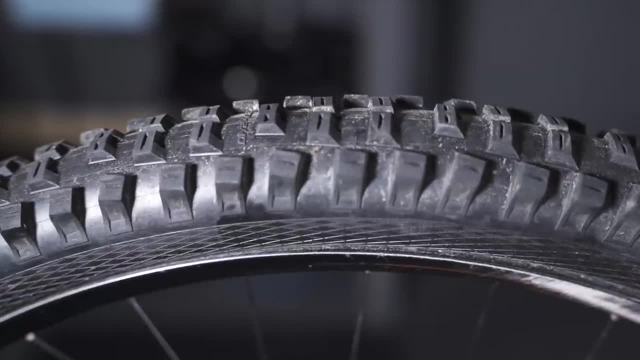 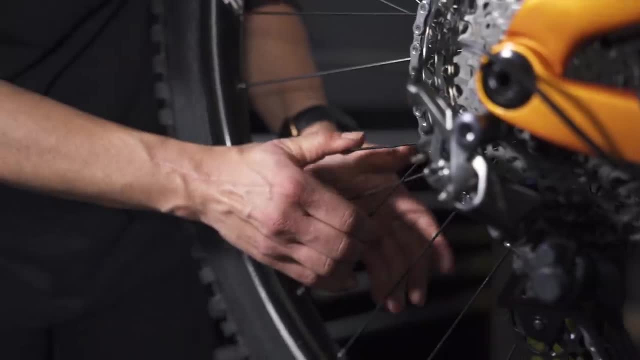 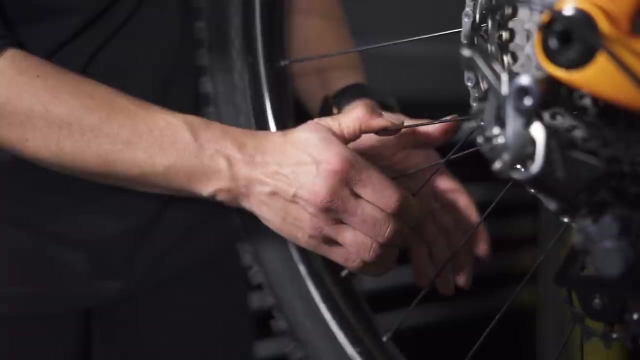 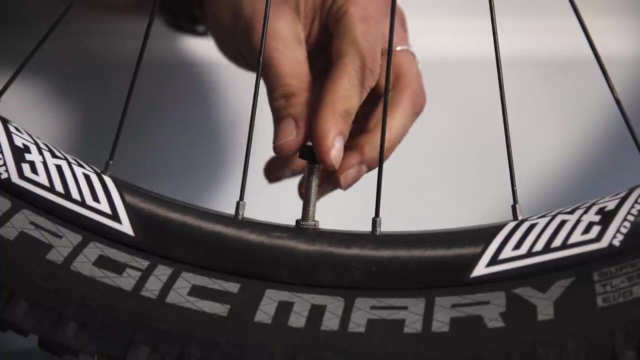 On the bike. I like to check the tread on the tire. Make sure you've got lots of nice, grippy tire tread for this time of year. Also a good time to just quickly check the spokes on your wheels. It's something that we don't look at often. Barely anybody touches those parts, but now's a good time. Just do a quick little finger tighten. Make sure everything's nice and snug When topping up the sealant and the tires. what I like to do is just use a little sealant bottle with a really small hole on the end, And then I will. 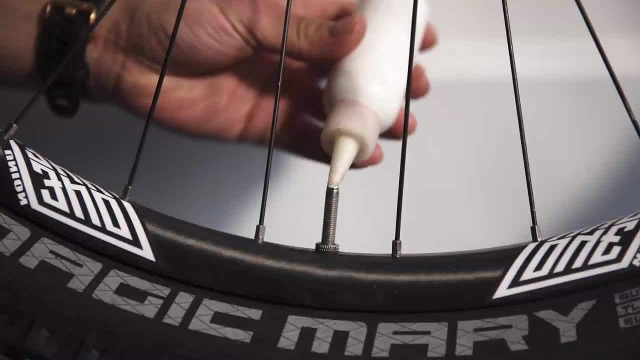 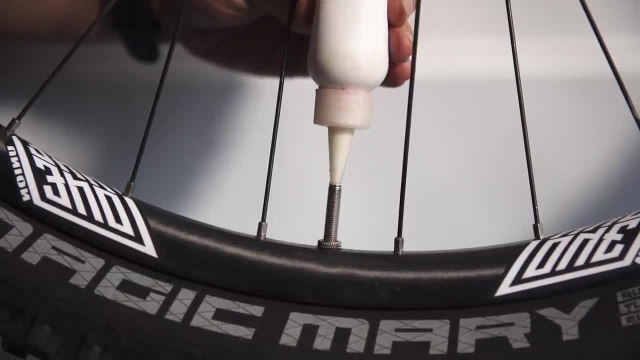 take out the valve core center and insert the sealant there. That method works really well for me. I don't have to rip the tire off the bead and the rim. I don't have to risk damaging the rim tape, because you know how frustrating that is. You just go to put a little bit of sealant in there And